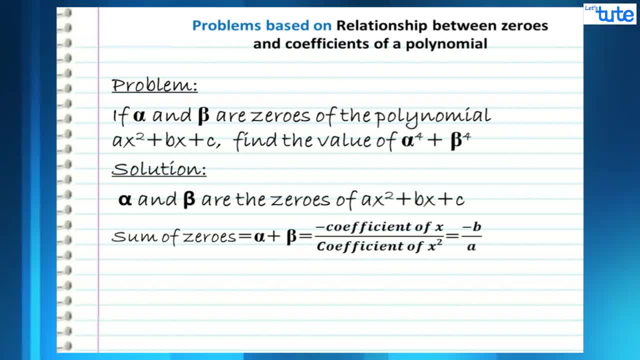 equal to minus coefficient of x upon coefficient of x square. In this case, coefficient of x is b, So minus b becomes our numerator, and coefficient of x square is a, So a becomes our denominator. So sum of the zeros is equal to minus b upon a. Similarly, product of the zeros is equal to alpha beta, which is given by constant term upon coefficient of x square. In this case, our 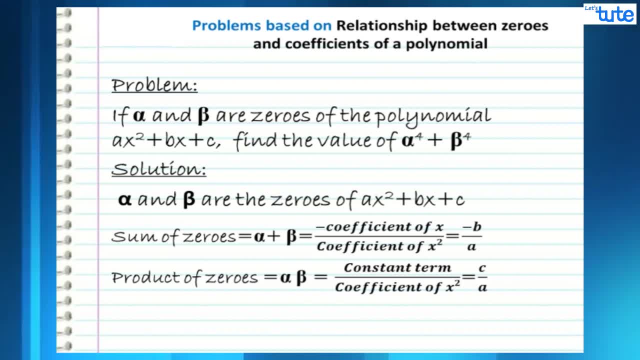 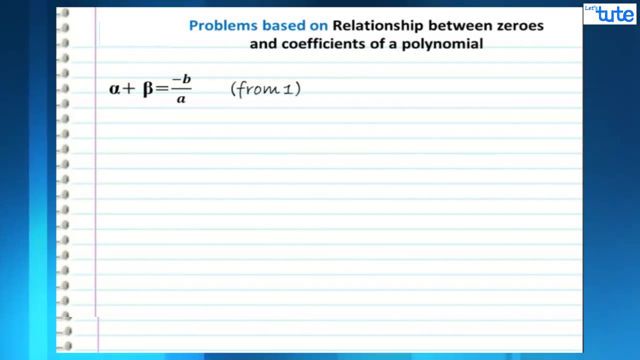 constant term is c, So c becomes our numerator, and coefficient of x square is a, So a becomes our denominator. Therefore, product of zeros is equal to c upon a. So we have: alpha plus beta is equal to minus b upon a from 1, and alpha beta is equal to c upon a from 2.. Now, using these two pieces of information, we have to find alpha raised to 4 plus beta raised to 4.. 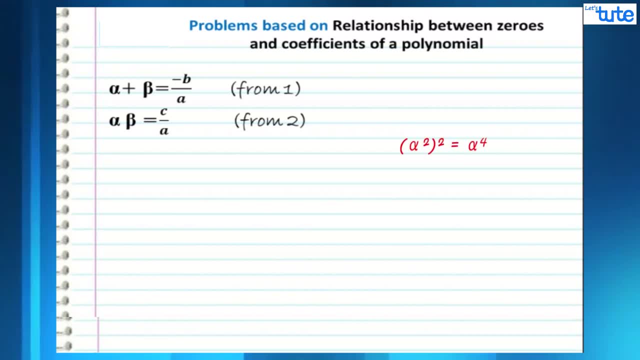 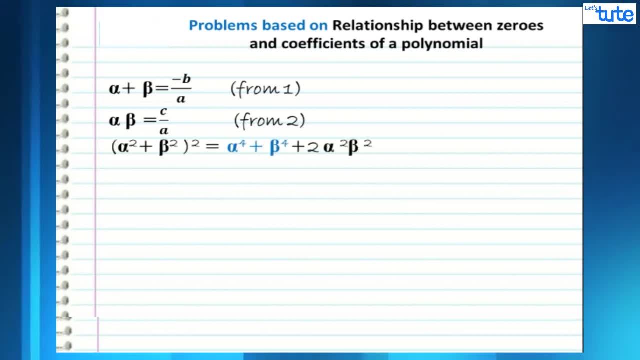 what is alpha square plus beta square- the whole square. We will get alpha square plus beta square. the whole square is equal to alpha raised to 4 plus beta raised to 4 plus 2. alpha square, beta square. Now how will we get alpha square plus beta square? in the first place, We can get alpha. 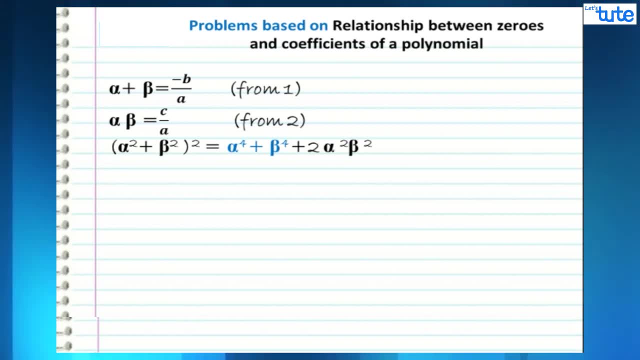 square plus beta square only if we take alpha plus beta the whole square. Remember the formula: a plus b, the whole square is equal to a square plus b square plus 2ab. we will use the same formula over here. so alpha plus beta, the whole square will give us alpha square plus beta. 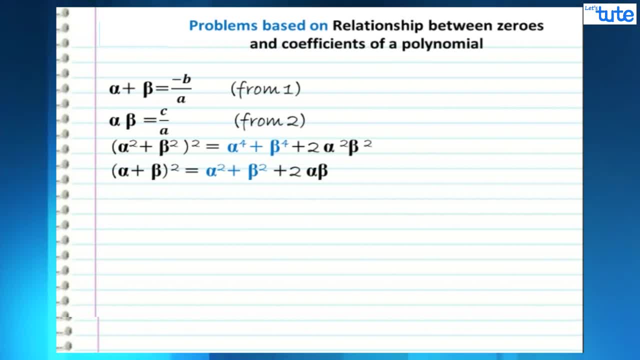 square plus 2 alpha beta. so now, using this equation, we will be able to proceed further. why? because we have the value of alpha plus beta and we have the value of alpha beta. now, putting these two values in this expression, we can find out the value of alpha square. 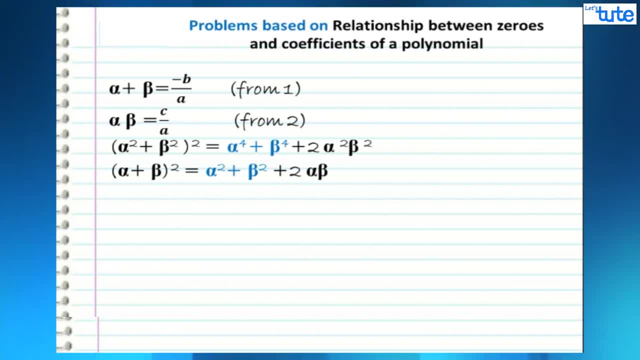 plus beta square, which can be eventually used to find out the value of alpha raise to 4 plus beta raise to 4. so after substituting the values we get minus b upon a. the whole square is equal to alpha square plus beta square plus 2.. 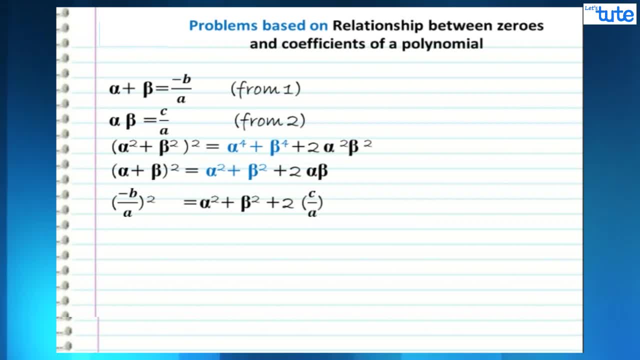 c upon a. now opening the bracket, we get b square upon a square is equal to alpha square plus beta square plus 2c upon a. taking 2c upon a on the left hand side, we get b square upon a square minus 2c upon a is equal to alpha square plus beta square. now check the. 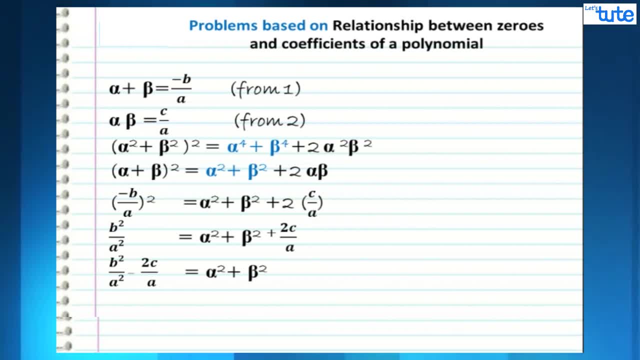 denominators of the LHS. the denominators are a and b square and a, so we'll have to take LCM. so upon taking LCM we will get b square minus 2 AC upon a square. so alpha square plus beta square is equal to b square. 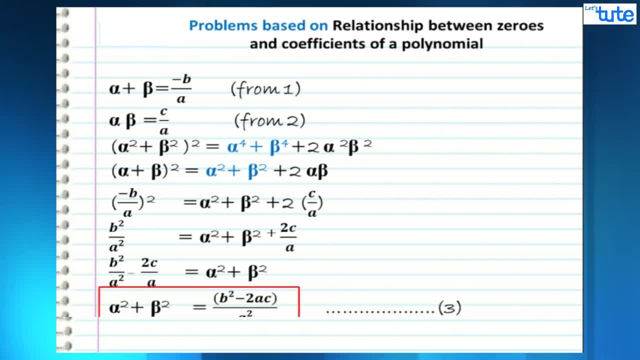 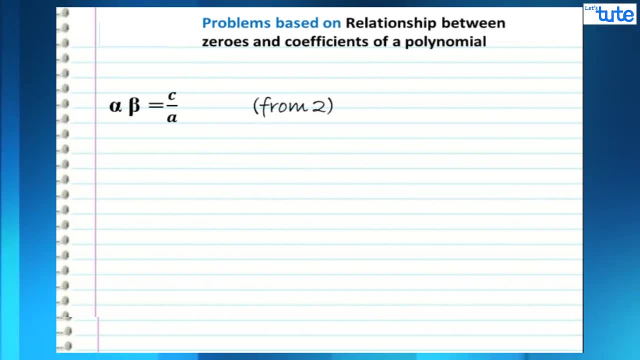 minus 2 AC upon a square. let us keep this as point number 3. now from point 2 we have: alpha beta is equal to C upon a and alpha square plus beta square is equal to b square minus 2 AC upon a square. from point number 3: using 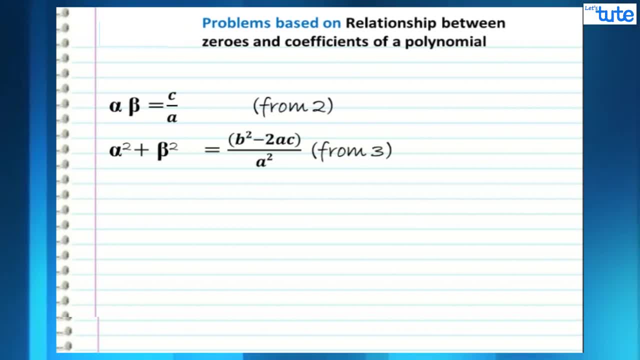 these two pieces of information. now we can find out the value of al dollar 2 times a box dollars plus b by the squareрат to m square plus 4, plus beta tends to 4. let's see how we will use the formula a plus b. the whole squared is equal to a square plus. 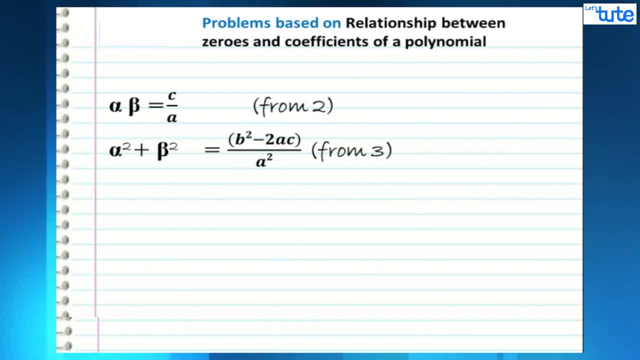 b squared plus 2 a b. q radar equals toive Motoрут. x2-2 b equal to e. x225難ать b square from t's x2–b square plus two a b square represents A and beta square represents B. 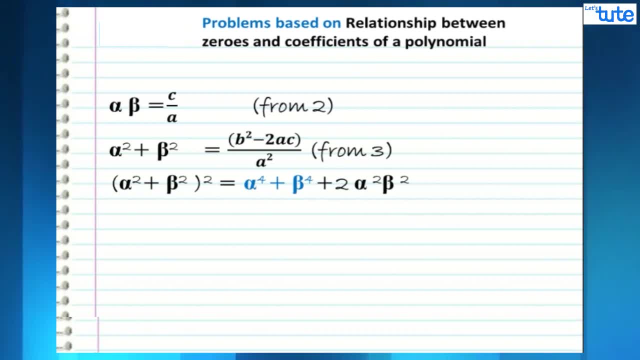 So the whole square is equal to beta raised to 4 plus 2 alpha square. beta square, which can also be written as alpha square plus beta square, the whole square is equal to alpha raised to 4 plus beta raised to 4 plus 2 alpha beta, the whole square. 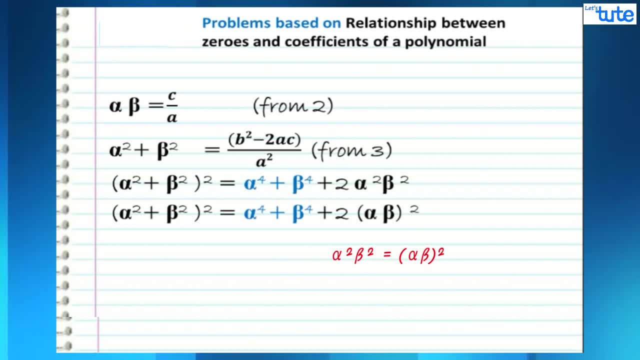 In this particular step, we have clubbed alpha beta together and we put them under the whole square. Check out here: from 3, we have the value of the LHS and we have the value of alpha beta from number 2.. So we are using this particular step. 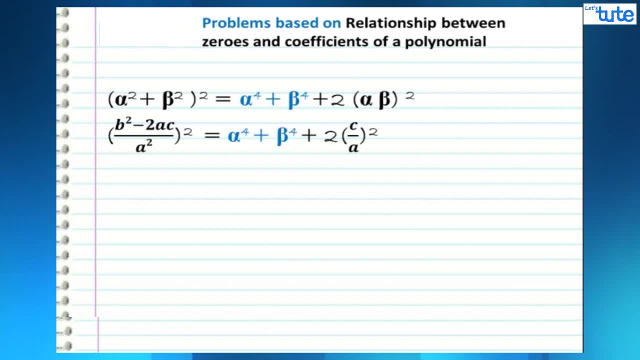 So on substitution we will get on LHS we will get b square minus 2ac upon a square, the whole square which was the value of alpha square from alpha square plus beta square is equal to alpha raise to 4 plus beta raise to 4 plus 2c upon a, the whole square which. 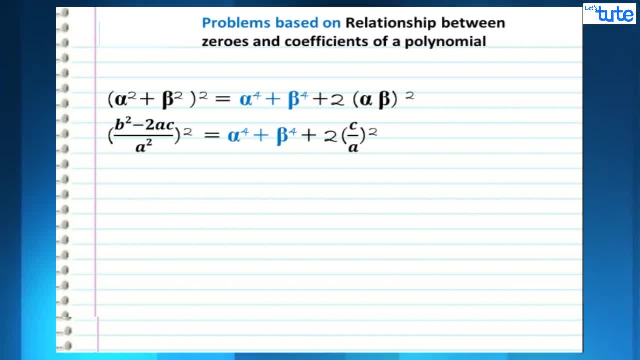 is the value of alpha beta. Now, upon opening the brackets, we get b square minus 2ac. the whole square upon a raise to 4.. Remember: a square, the whole square, will give us a raise to 4.. So our LHS becomes b square minus 2ac. the whole square upon a raise to 4 is equal to. 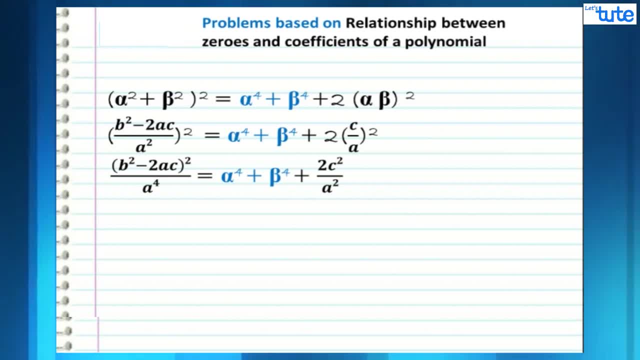 alpha raise to 4 plus beta raise to 4 plus 2c square upon a square. Now, taking 2c square upon a square on the left hand side, we get b square minus 2ac. the whole square upon a raise to 4.. 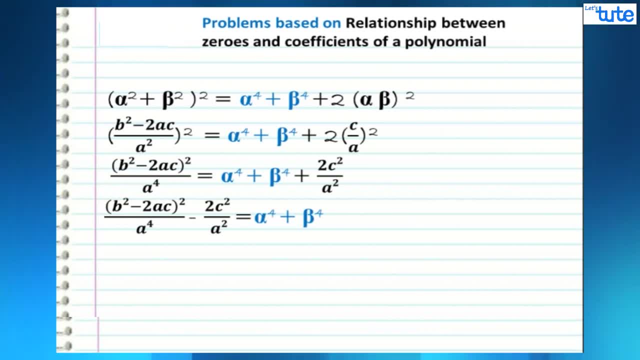 minus 2C, square upon A square which is equal to alpha raised to 4 plus beta raised to 4.. Now check, in this step, the denominator of this term is A raised to 4 and of this term is A square, So we will have to take LCM. So, upon taking LCM, we get B square minus 2AC, the whole. 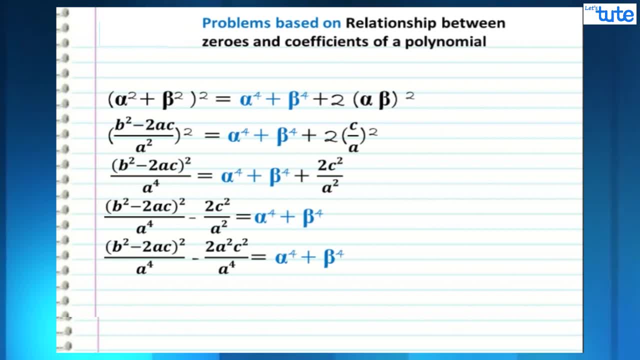 square upon A raised to 4 minus 2A. square C: square upon A raised to 4, which is equal to alpha raised to 4 plus beta raised to 4.. So, finally, alpha raised to 4 plus beta raised to 4 is equal. 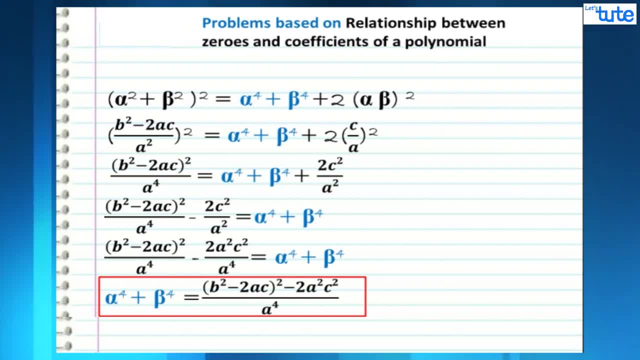 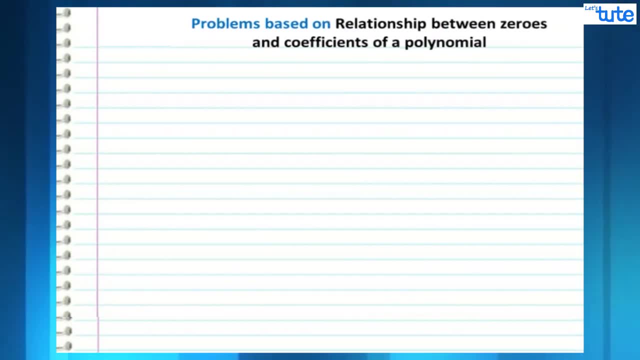 to B square minus 2AC, the whole square minus 2A. square C square upon A, raised to 4.. Let's see our second problem. Second problem says: if alpha and beta are zeros of the polynomial AX square plus BX plus C, find the value of alpha cube plus beta cube. 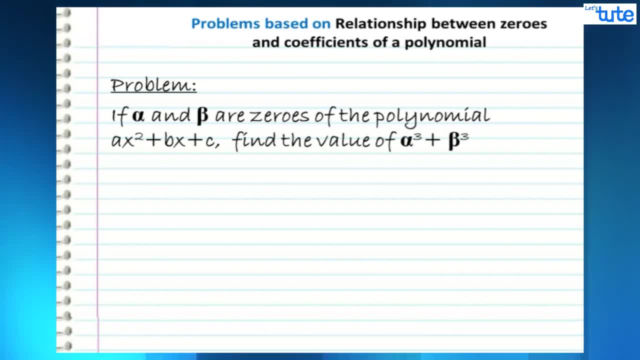 This is similar to our first problem, except that over here they have asked us to find the value of alpha cube plus beta cube. So let's see how to solve this problem Here. alpha and beta are the zeros of AX square plus BX plus C, and the sum of the zeros can be given as alpha plus beta, which. 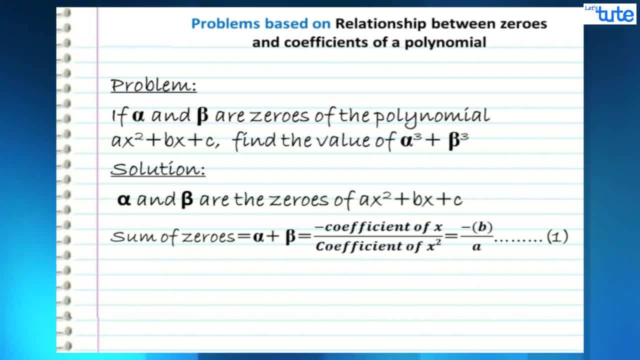 is minus 0. It is an equation of a coefficient of x upon coefficient of x square. In this case the coefficient of x is B, So our numerator becomes minus B and the denominator becomes A, So sum of zeros is equal to minus B. 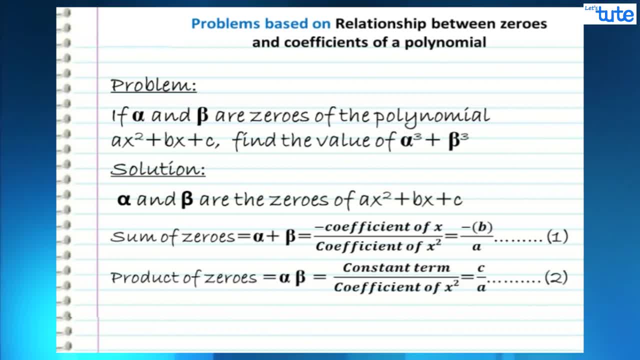 upon A. Let us keep this as equation 1. and a. product of zeros is equal to alpha beta, which is constant term upon coefficient of x square, which is equal to C upon A. So product of zeros is to c upon a, because constant term in this expression is c and coefficient of x square. 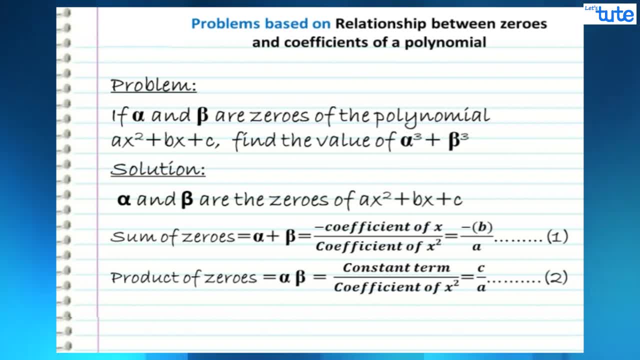 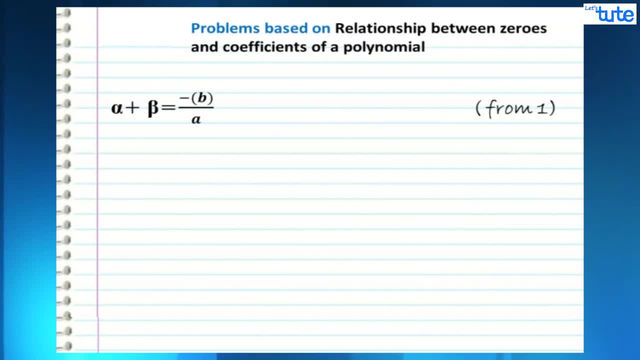 is a, So product of the zeros is equal to c upon a. Let's keep this as point 2.. Now we have two pieces of information. We have: alpha plus beta is equal to minus b upon a from 1. Alpha beta is equal to c upon a from 2.. What do we do with this information? We 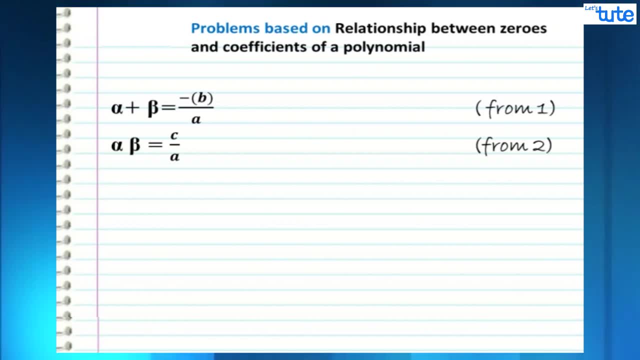 will use this information to find alpha cube plus beta cube. Now how are we going to get alpha cube plus beta cube? We will get alpha cube plus beta cube only if we take cube of alpha plus beta. So alpha plus beta, the whole cube is equal to alpha cube plus beta cube.